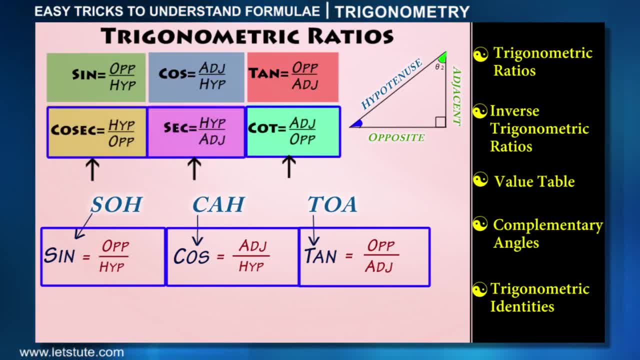 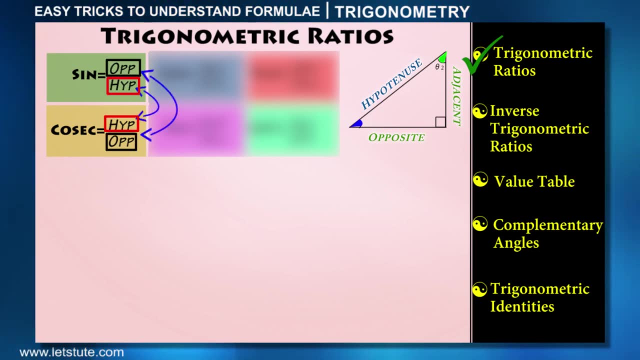 trigonometric ratios and to get the rest three we need to just reverse these ratios. Thus we get cosec, sec and cot. Now, if we observe, sine and cosec has the same elements in their ratio and cosec can be obtained just by inverting the sine ratio. Therefore the multiplication 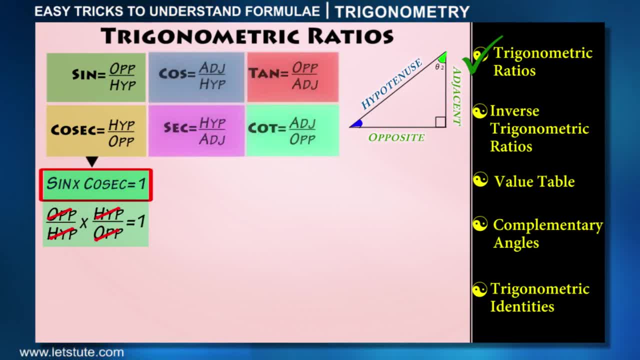 of sine and cosec is 1.. Similarly, when we reverse the cos ratio, sec is obtained, And so multiplication of sec and cos is 1.. And same goes for tan and cot, And therefore the pairs sine cosec, sec, cos, tan, cot are: 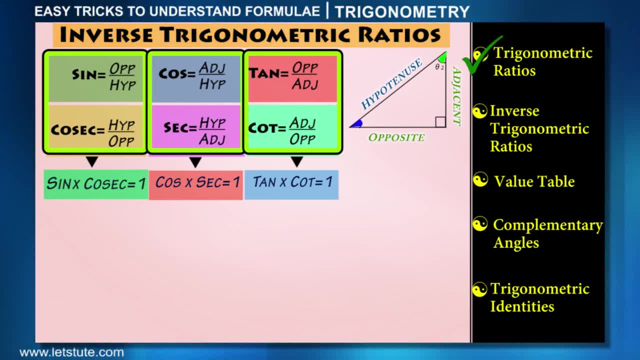 called inverse trigonometric ratios. So further we write sine as 1 upon cosec, or cosec is equal to 1 upon sine. Same way, cos is equal to 1 upon sec and sec is equal to 1 upon cos And tan is equal to 1 upon cos And tan is equal to 1 upon cos And tan is equal to 1 upon 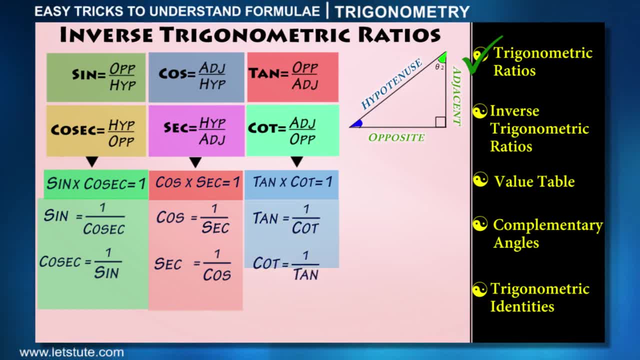 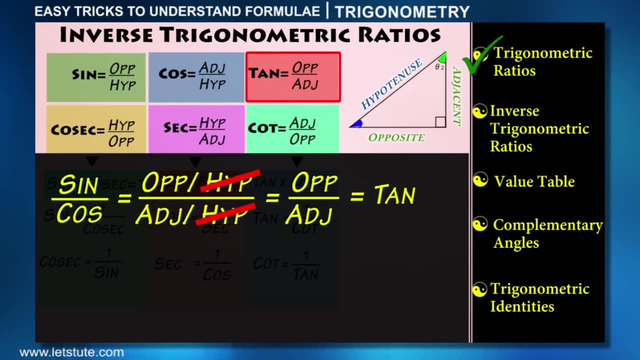 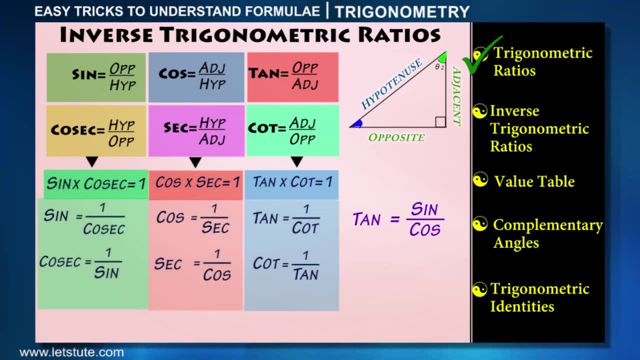 1 upon cot, cot is equal to 1 upon tan. Now if we take the ratio of sine and cos, we get the same ratio as tan. Thus we have got one more formula, that is, tan is equal to sine upon cos. and since tan and cot are inverse, cot is equal to cos upon sine. So you see, 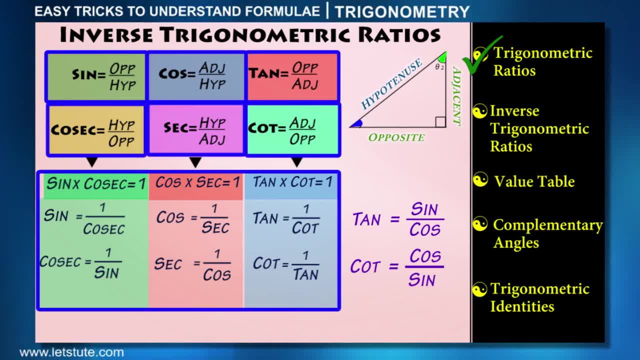 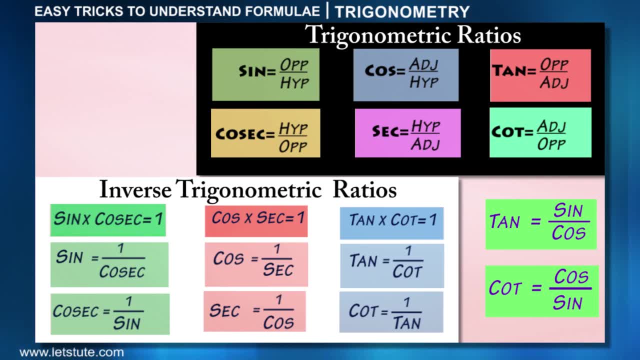 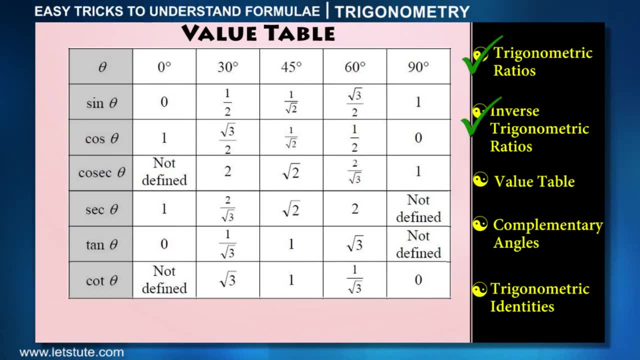 by just simply paying with this six trigonometric ratio, we can derive the different formulae. Let's summarize the formulas we learnt till now. Now we proceed to the next. So we are going to see a small trick to remember this value table for standard angles: 0,, 30,, 45,, 60 and 90 degrees. These values are very important. 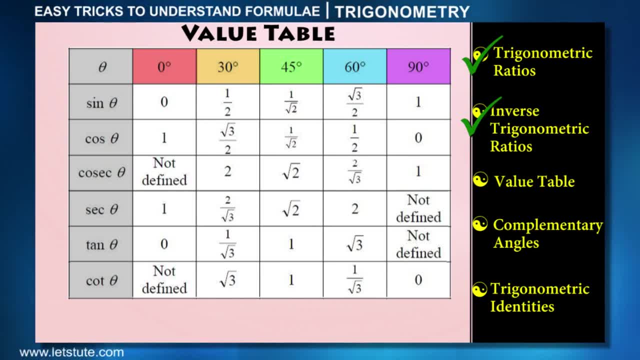 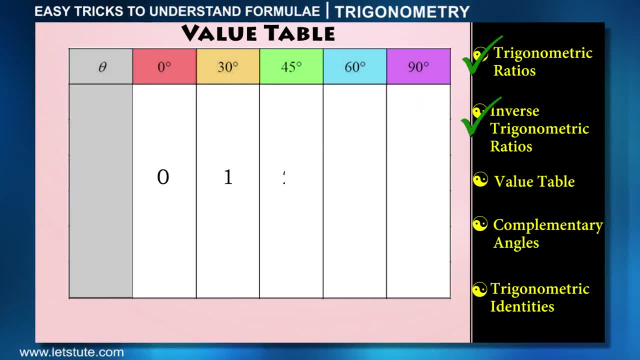 and we often use them. use them in solving trigonometric questions. So to build this entire table, we first write down the numbers from 0 to 4 in below these angles, Now divide each of them by 4, then take the square root And this is the value for our very first trigonometric ratio sine. 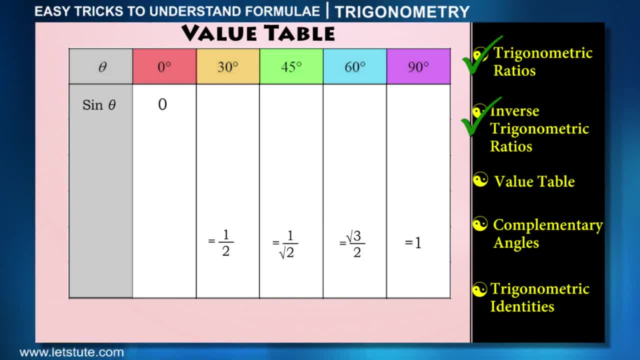 We read it as sine 0 is 0,, sine 30 is 1, and so on to sign 0.. Now recall: we have already learned this trick, and its logical explanation too, in our one of the sessions. So if you, 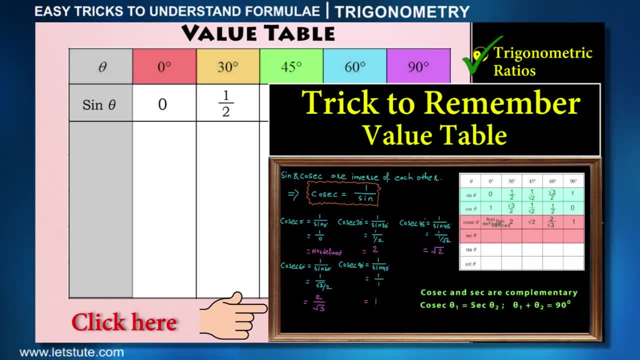 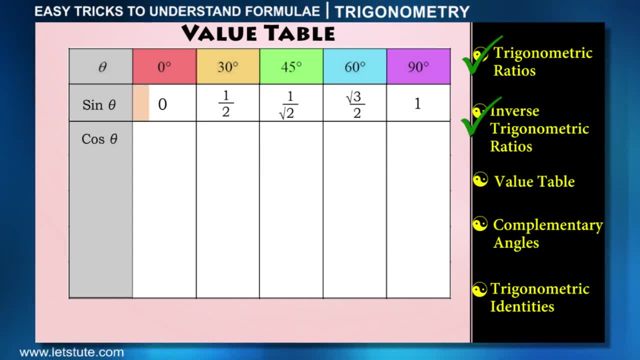 wish to watch that particular session, you may click here. So, after getting the values for sine, we get the values for cos by simply writing this: values in reverse order. Remember that the value for sin is half. Thank you, Have a good day. 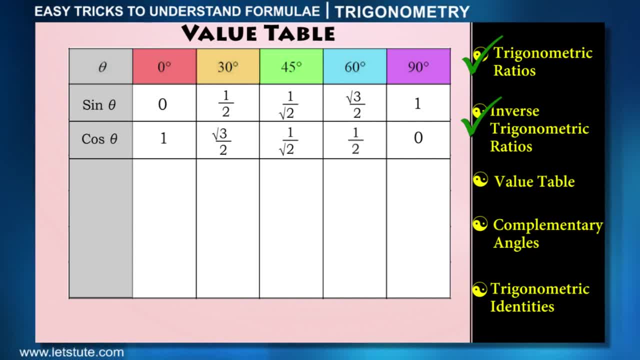 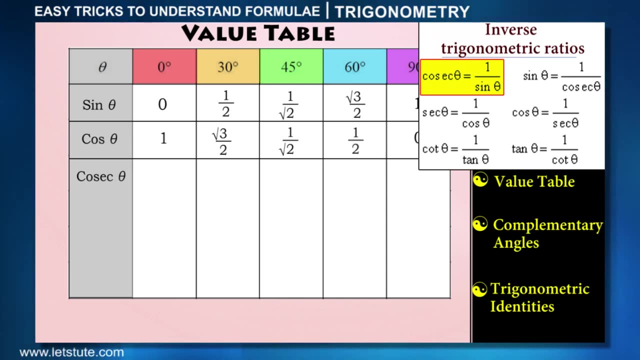 be values for sine and cos. we use the concept of inverse trigonometric ratios to get the further values. So, as we know, sine is inverse of cosec and vice versa. so the value for cosec 0 will be equal to 1 upon sine 0, that is not defined. Cosec 30 will be equal to 1 upon 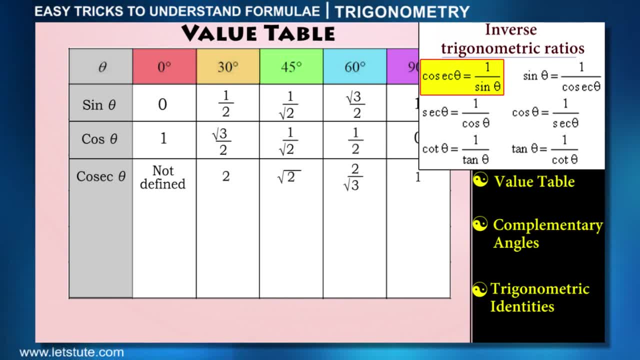 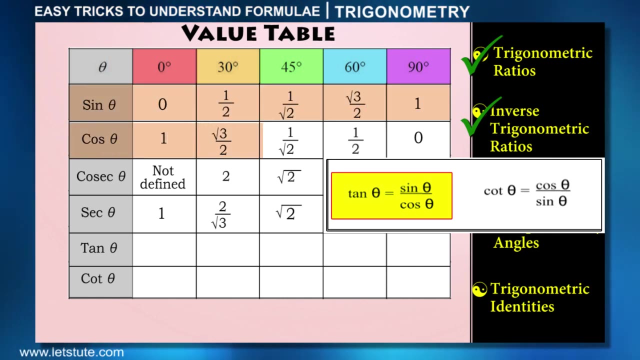 sine 30, that is 2, and like this you will get all the values for cosec 2.. Next, we know sec is inverse of cos. so similarly, sec can be obtained by inverting the cos ratio. Now only tan and cot are left, and we also know that the ratio of sine and cos is tan. so we divided. the value of sine by the value of sin. Cosec 30 is inverse of cosec 2, as you can see in the right side of the equation, it is quite obvious that this is inverse 하. there is only tan and cot left and only tan and cos saws. So we divide the value of sine by the value of sine by the. 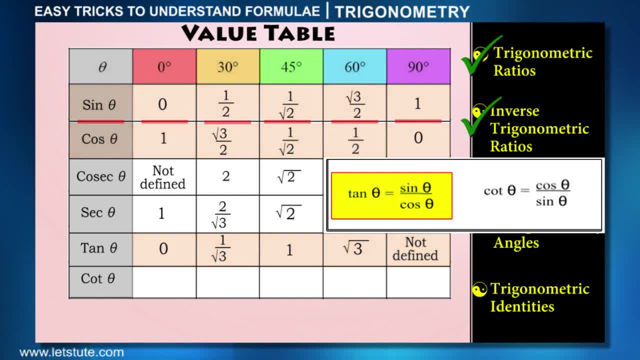 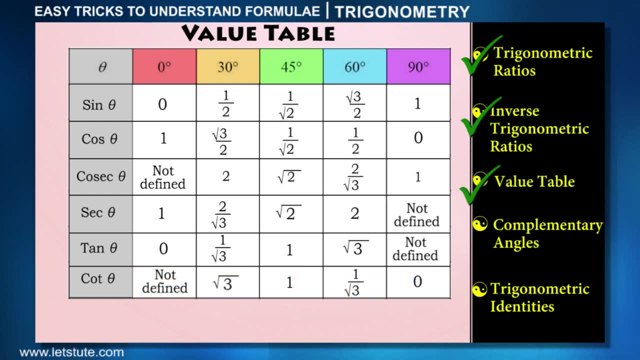 cos to get the values for tan. Tan and cot are inverse trigonometric ratios. so once again, by flipping the tan ratio we get the values for cot And you can see. the value table is completed. I hope this was easy for you. We know a right angle triangle has one fixed. 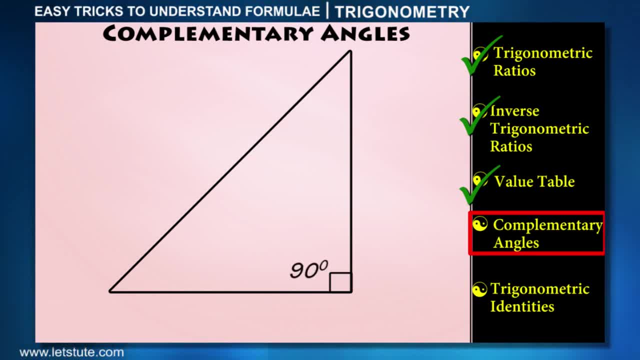 angle of 90 degrees. So it is very much obvious that the sum of the rest two angles must be 90 degrees. Therefore those two angles are called complementary angles because they complete a triangle. Let's now give some values to its sides- x, y, z- And we also write the six. 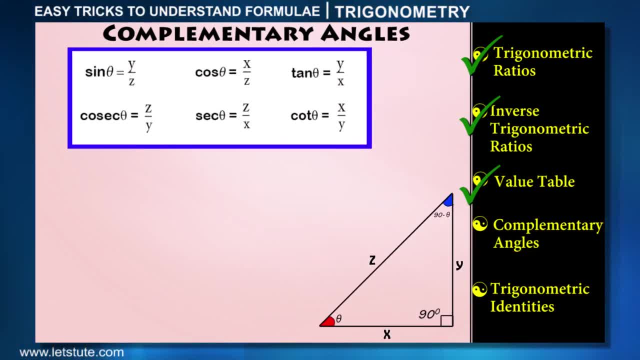 trigonometric ratios for both the angles theta and 90 minus theta. So what we observe here? We observe that the value for tan is 90 degrees and the angle for cot is 90 degrees. So what we observe here? We observe that the value for tan is 90 degrees and the angle for cot is 90 degrees. So what we observe here? We observe that the value for 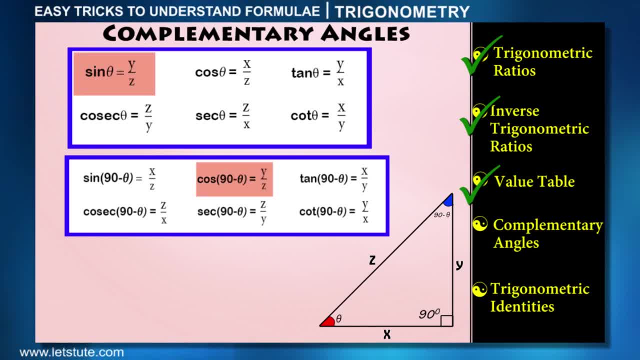 sin theta and cos 90 minus theta are same, Then cos theta and sin 90 minus theta are equal. Similarly, the value of tan theta and cot 90 minus theta are equal. cot theta and tan 90 minus theta are equal. The same thing happens with cosec and secto, So understand. 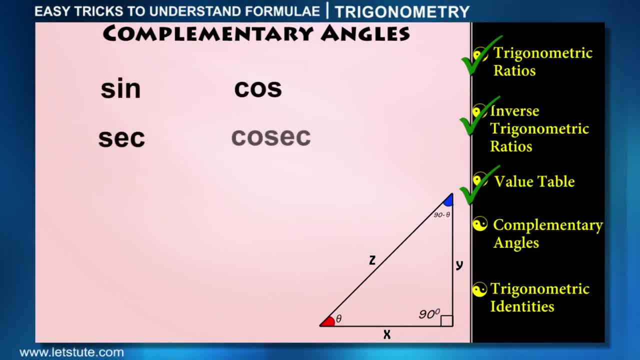 that sin, cos sec, cosec and cos 90 minus theta, equal Interesting right. And when you forget, tan cot, these pairs are equal for the two angles whose sum is 90 degrees, and hence these pairs are called complementary. and these complementary pairs we can never forget, because we have to just add co of the word. 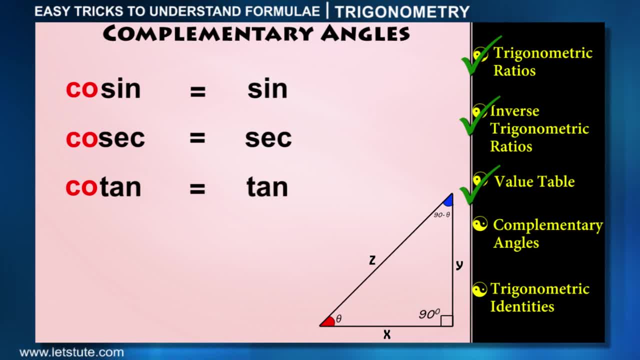 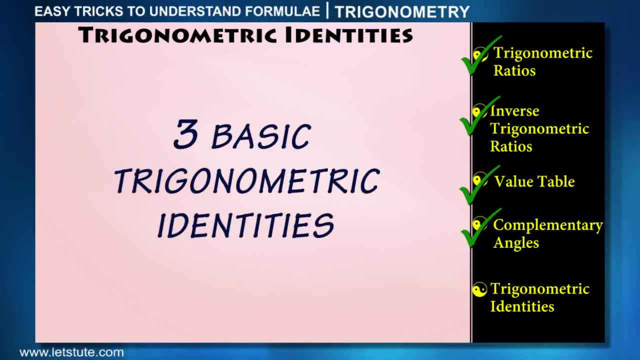 complementary before sine, second and tangent. now, next thing that we are going to learn is about the three basic trigonometric identities. Pythagoras theorem is the very first step in getting these three. so in this right-angle triangle, if we apply Pythagoras theorem, we write hypotenuse: 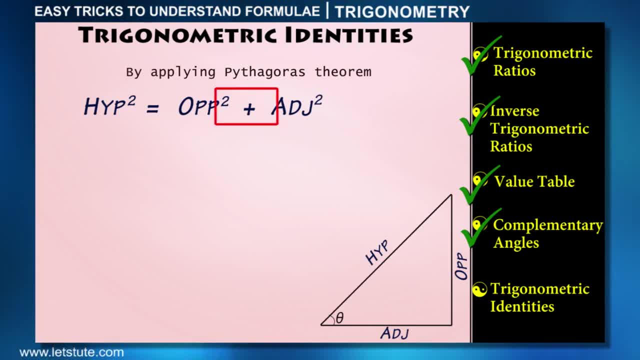 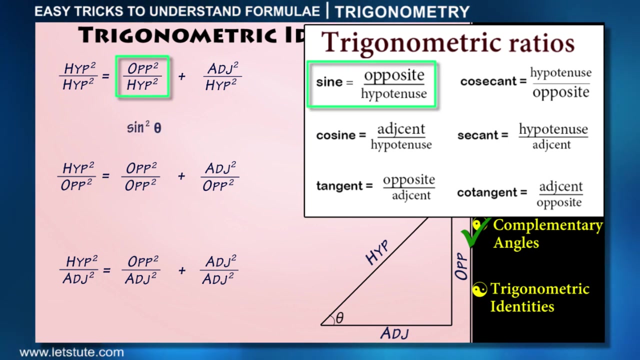 square is equal to opposite side square plus adjacent side square. divide these twice, once by hypotenuse square, then by opposite side square, and then by adjacent side square. and now, as we already know that this ratio is defined as sine, this is cos, and then cosec, cot, sec and tan. so, friends, since Pythagoras theorem is the initial, 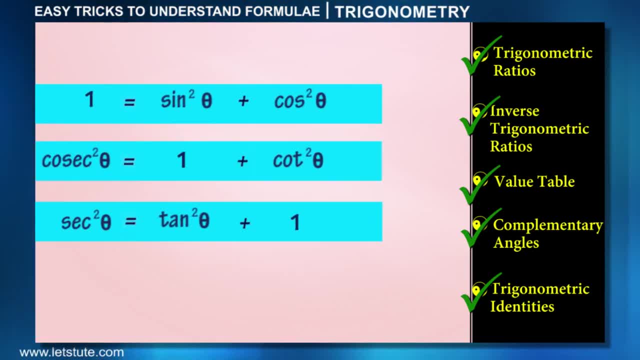 step in getting these three identities. these are also called Pythagorean identities and, like all the other Pythagorean formulae of trigonometry, these three are also very important in solving trigonometric questions and they are very easy to remember because once we know that sine square theta plus cos square theta is one, then to obtain the 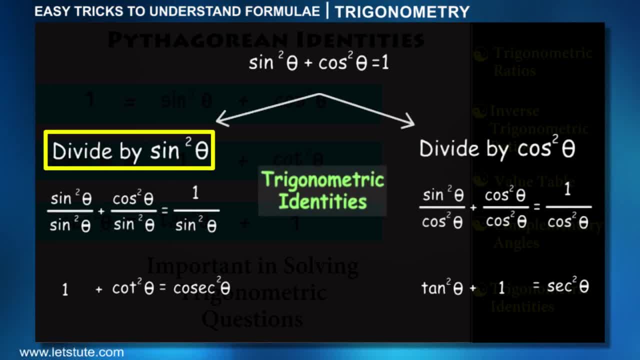 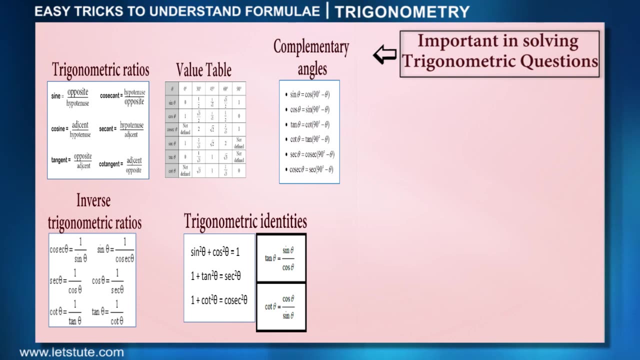 other two. we divide this identity first by sine square theta and then by cos square theta. so all the formulae that we learned till now is very helpful in solving the trigonometric questions, especially the identities. but in trigonometry there are word problems too, which are also equally important, and to solve them correctly, along with this formulae, we should also understand few basic terms like horizontal level, line of sight angle of elevation and depression. let's understand each of these in more simpler terms. so when we look straight ahead, we can see that there is a line of sight angle of elevation and depression. let's understand each of these in more simpler terms. so when we look straight ahead, we can see that there is a line of sight angle of elevation and depression. let's understand each of these in more simpler terms. so when we look straight ahead, we can see that there is a line of sight angle of elevation and depression. let's understand each of these in more simpler terms. so when we look straight ahead, we can see that there is a line of sight angle of elevation and depression. let's understand each of these in more simpler terms. so when we look straight ahead, we can see that there is a line of sight angle of elevation and depression. let's understand each of these in more simpler terms. so when we look straight ahead, we can see that. 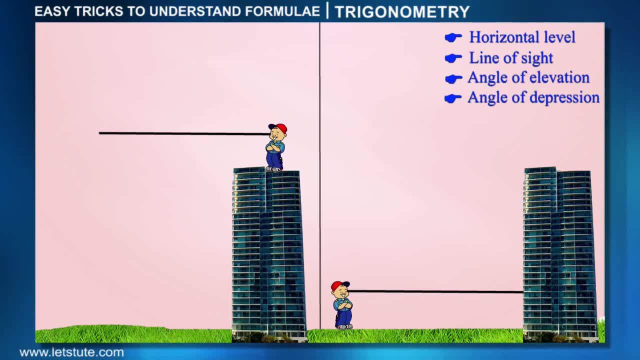 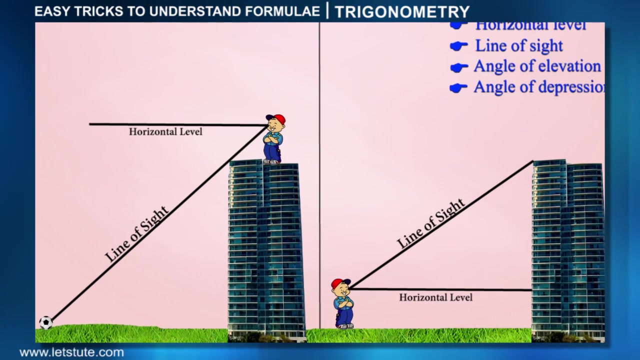 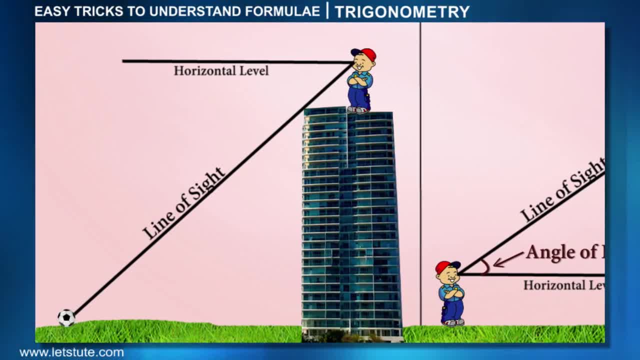 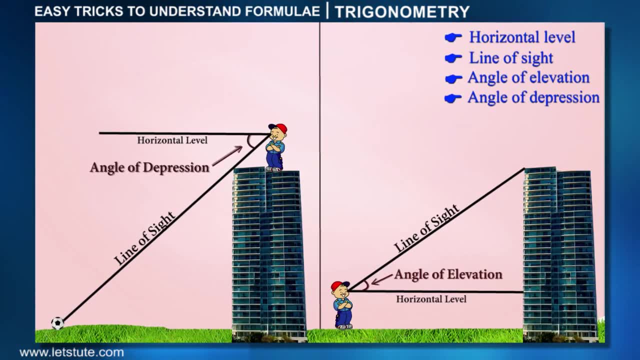 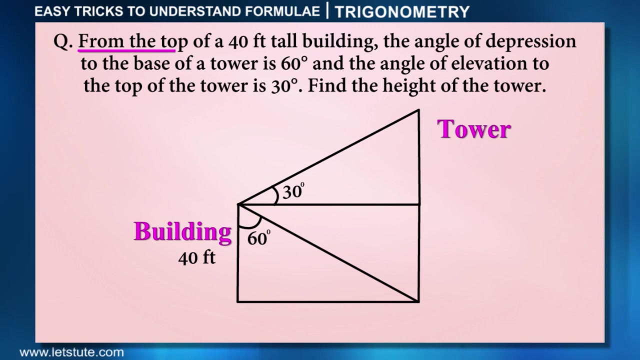 when we look down, the angle made by the line of sight with the horizontal level is the angle of depression. So, friends, this basic knowledge helps us in drawing accurate diagrams while solving word problems. So look at this question and its diagram From the top of. 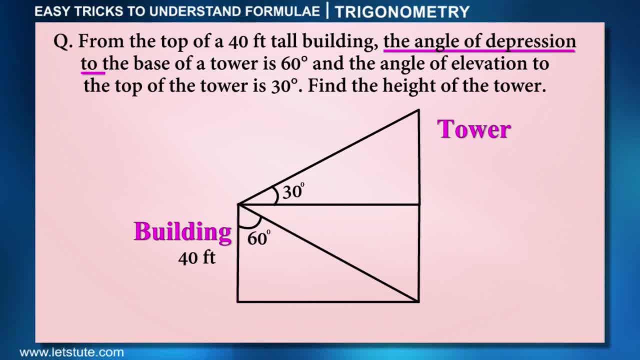 a 40 feet tall building, the angle of depression to the base of a tower is 60 degrees and the angle of elevation to the top of the tower is 30 degrees. Find the height of the tower. So in this diagram AB is considered as the building, EC as tower. But my question is: is